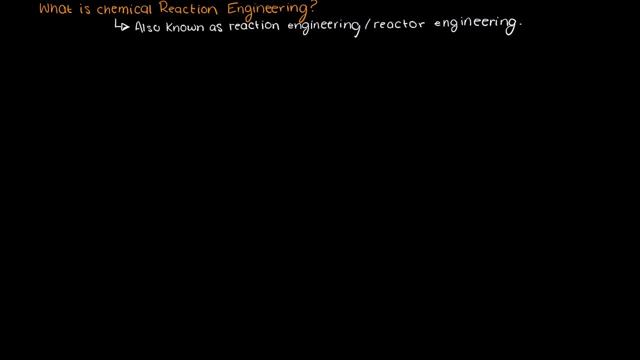 Ok, so what exactly does chemical reaction engineering mean, and what would you be learning in this course? Well, as you may have imagined, chemical reactions are certainly going to be involved, and, in particular, the chemical reaction engineering course here is related to designing various chemical reactors to create the conditions. 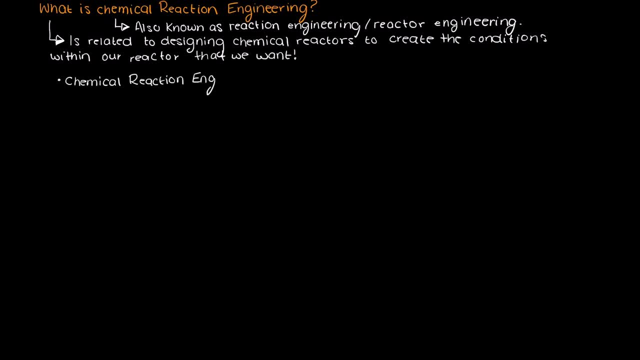 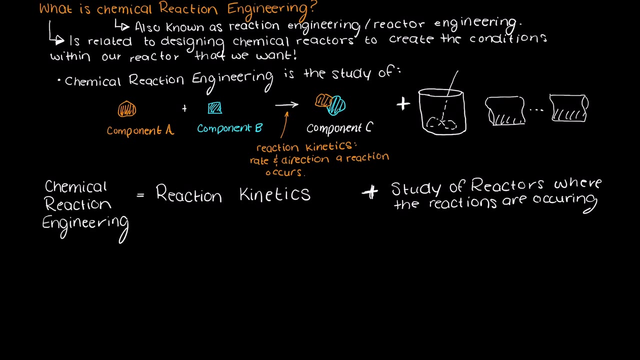 within a reactor that we want. So said more formally, chemical reaction engineering is basically the study of reaction kinetics, the rate and direction at which a reaction occurs, and the study of the reactors in which the reactions actually take place. By that I mean, let's say that we want to produce 80 kg of some product per hour. what? 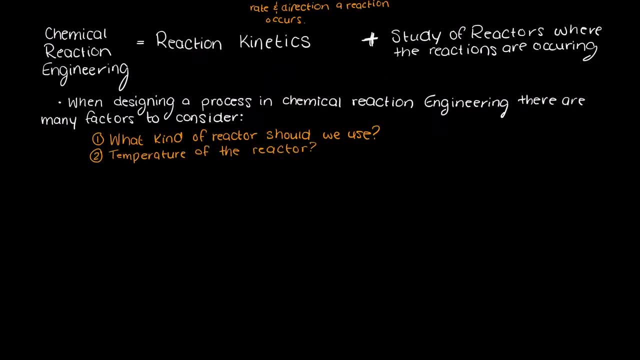 kind of reactor should we use? What temperatures should the reactor be at so that it doesn't explode or injure someone? Is there a safer or cheaper way to synthesize this product? These are just a few of the many questions the engineers who design the reactors must. 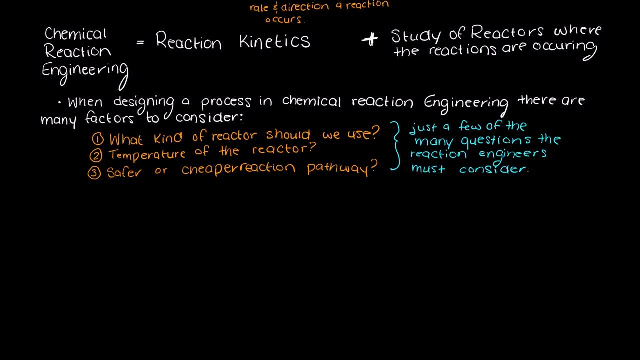 consider To build on what I previously stated. the primary focus of chemical reaction engineering is the study of the reactor design, such as: will a certain exothermic reaction melt our reactor due to the sheer amount of thermal energy generated? Economics are also a huge. part of this, as there is no point in developing a reactor that doesn't have a chemical reaction. The main focus of chemical reaction engineering is the study of the reactor design, such as: will a certain exothermic reaction melt our reactor due to the sheer amount of thermal? 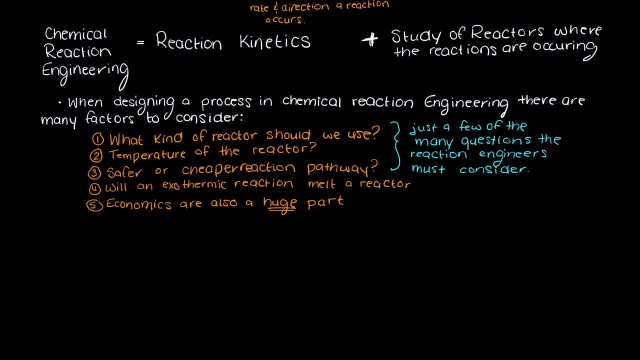 energy generated. In some cases, the reactor design and the chemical reaction design itself makes the chemical reaction not feasible to the investors or company putting in the money. In this case. the first question is: so how do we scale a process? By this I mean, how do we take the process we developed on a small scale, like a pilot? 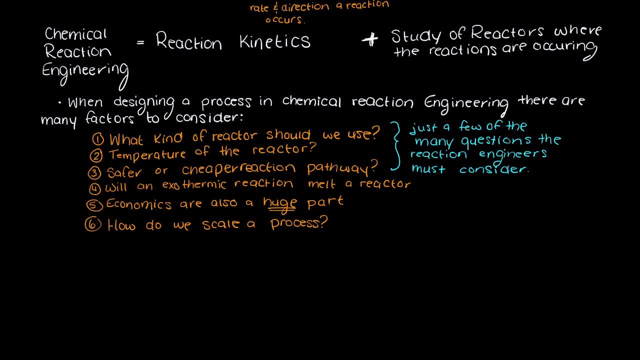 scale and scale it to be used in an industrial setting. So, now that we have an understanding of what chemical reaction engineering is, why is it important to learn about? Well, if you're watching this video, you're likely an engineering student: engineering. 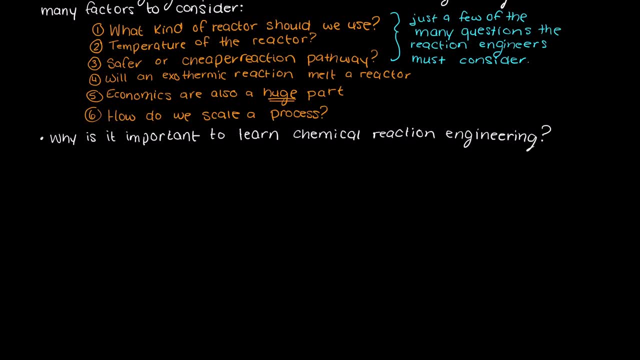 professional or someone else interested in chemical reaction engineering, interested in learning about reactor engineering. but why is it important? Well, learning about the relationship between reactors and chemical reactions is vital to developing processes that are not only safe but also cost effective- so think heating and cooling costs- and has minimal.